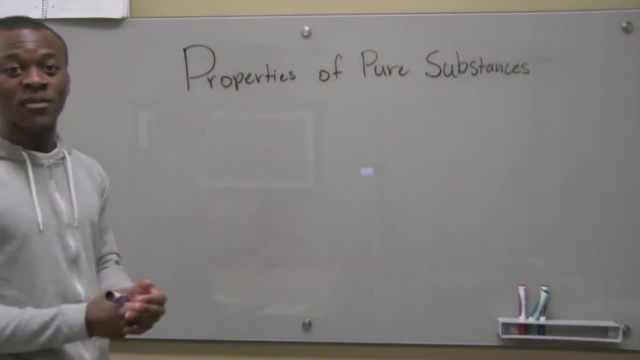 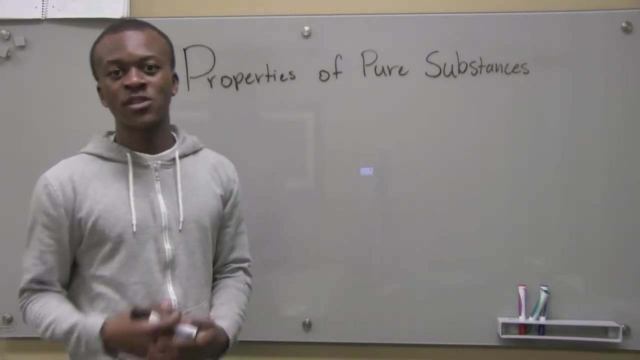 Hello everybody. Today we're going to be talking about properties of pure substances. Now, I'm sure we all have a good idea of what a pure substance is, but I'm going to try and go a little bit more in depth so we have a better understanding by the end of the video. Now, a pure substance is. 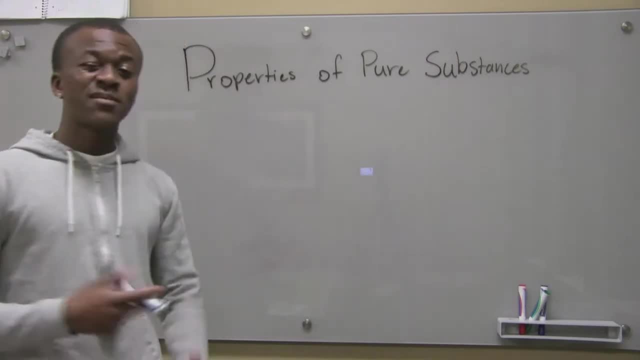 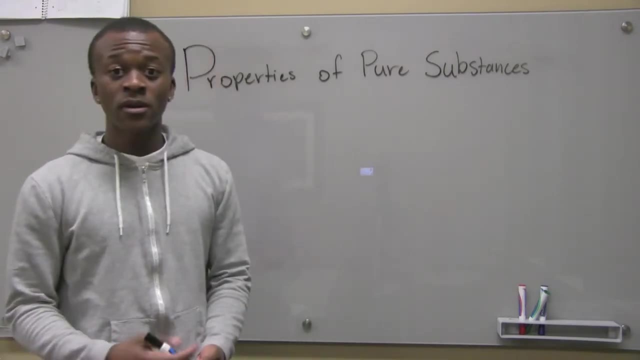 a substance that has a fixed chemical composition throughout. It's important to note that a pure substance might be composed of more than one chemical. So, for example, helium is a pure substance, right, But water can also be considered a pure substance. Water is made of both hydrogen. 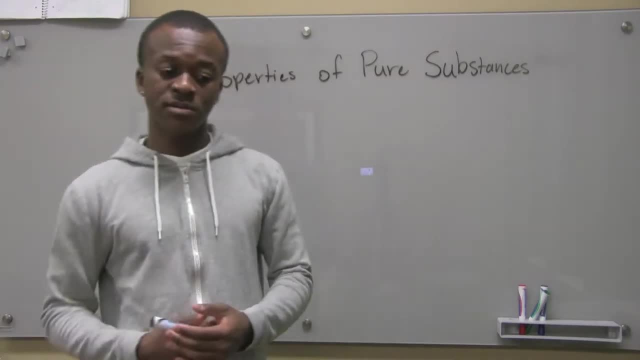 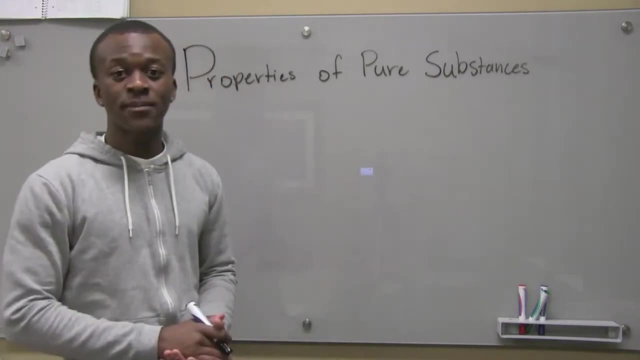 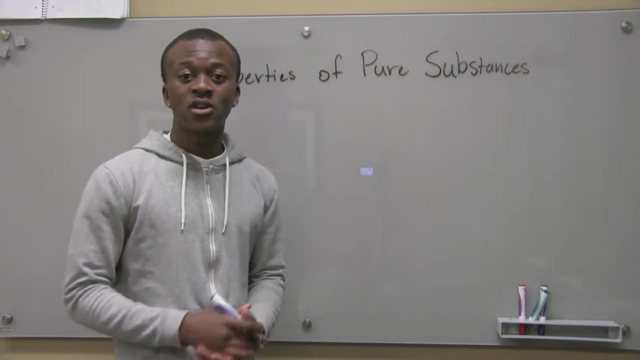 and oxygen, so that can also be considered a pure substance. It's also important to note that a pure substance can also be in more than one state, So ice water, for example, is an example of a pure substance. Ice water has both solid water and liquid water inside of it, so it's still considered. 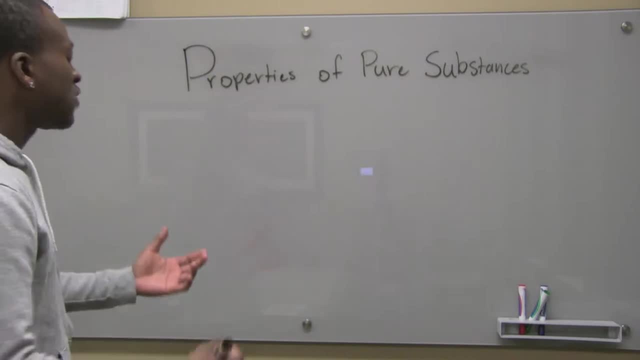 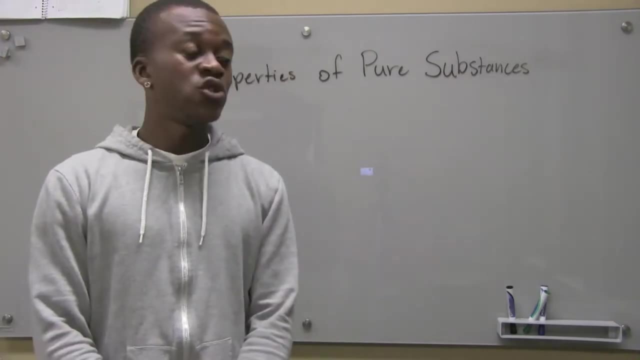 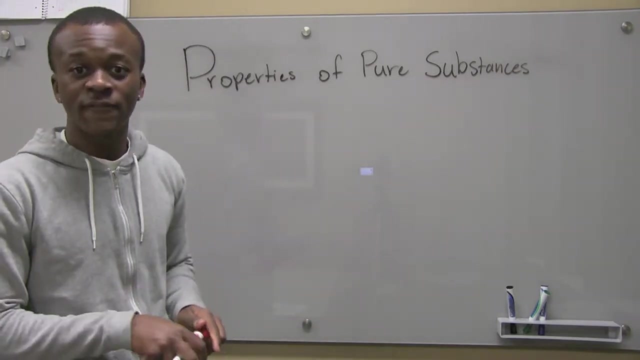 a pure substance. Now I'm going to give you guys some vocabulary that I want you all to know What I'm talking about. If I say things like compressed liquid or superheated vapor or a saturated liquid gas mixture, I want you guys to know exactly what I'm saying and not be confused. 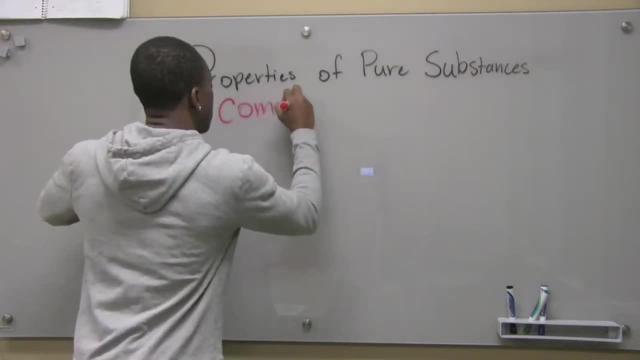 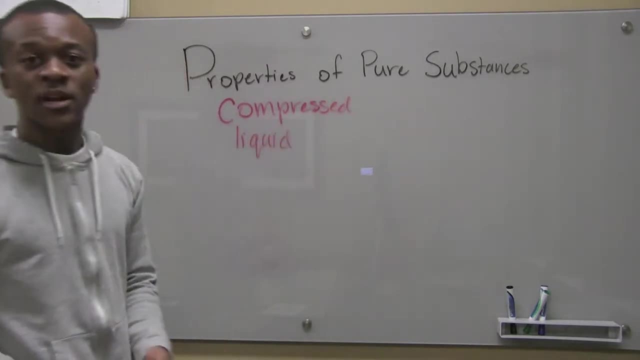 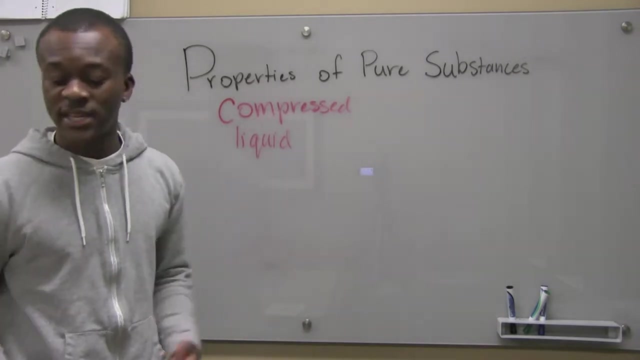 So if I talk about a compressed liquid, I'm talking about a liquid that has not yet undergone boiling right. This liquid is not in saturation, as you're going to see In the next example. that brings me to the term saturation. 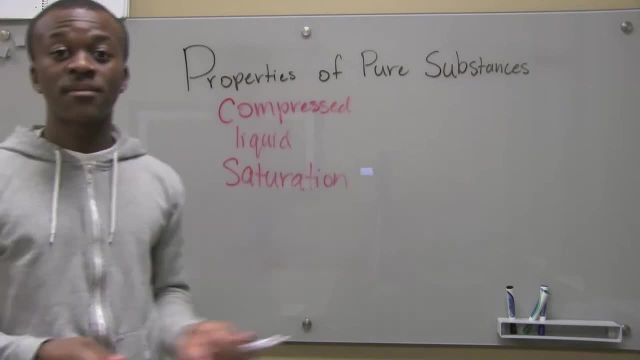 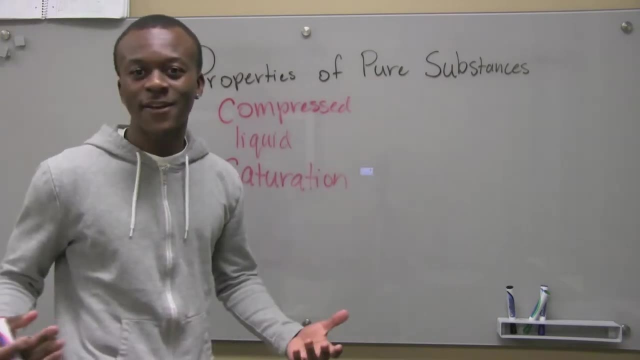 When I say something is undergoing saturation, I'm talking about boiling. I'm not talking about the type of boils you have on your face. I'm talking about like boiling. like you know, when we boil water on a kettle and it turns into steam, right, Or it turns into hot. 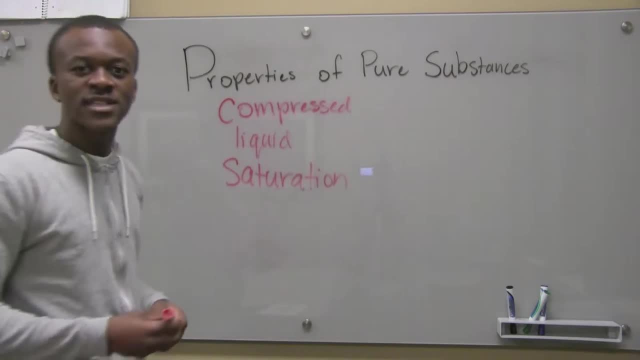 water and then you can see steam coming out of it. That's an example of like saturation, And in saturation we're going to find that we have more than one type of liquid. So if I say something is undergoing saturation, I'm going to find that we have more than one phase going on sometimes. 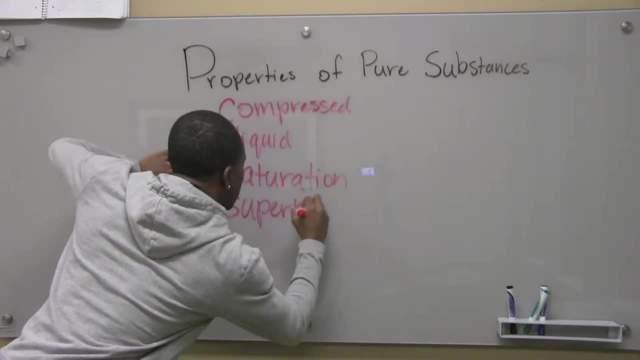 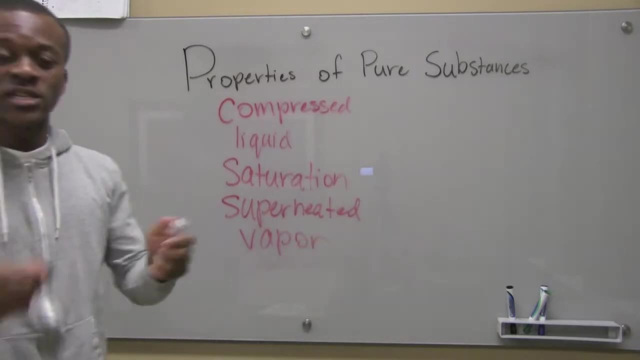 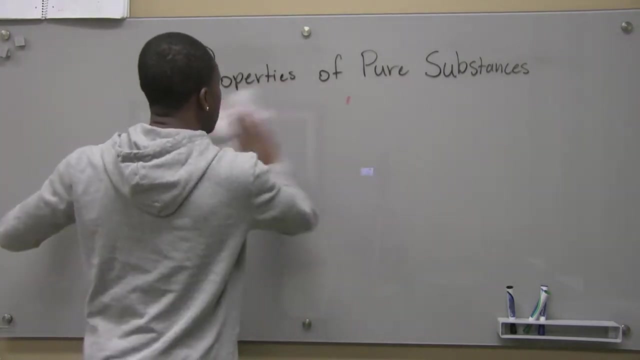 If I talk about a superheated vapor, I'm talking about a substance that has completely undergone boiling and finished boiling, So it's no longer boiling and it's completely a gas. It's an everyday gas that we know. So that's what I'm talking about when I say a superheated vapor. Now I'm going to draw something. 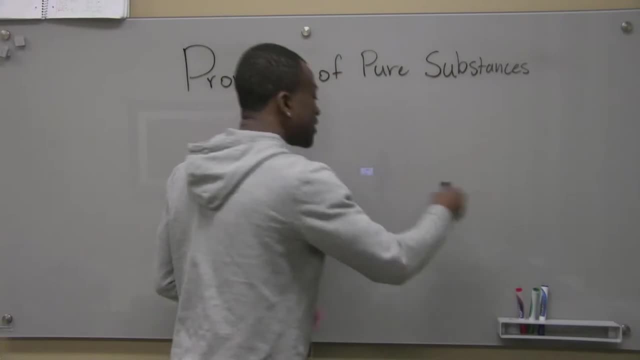 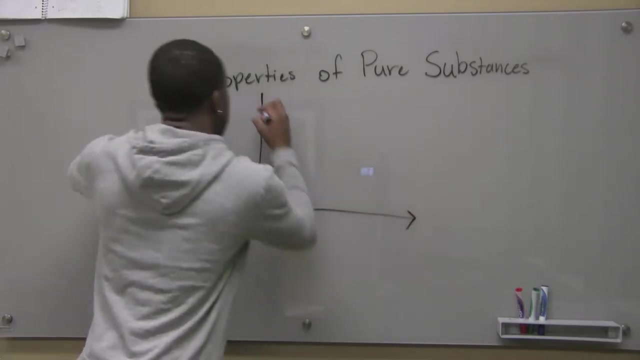 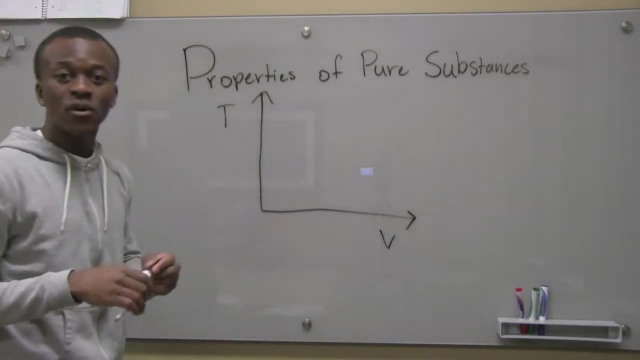 for you guys called a T-V diagram. The T stands for temperature and the V stands for volume or specific volume. Now, what we need to know with this is that this is temperature, this is volume or specific volume, Something I'm going to draw like an example of. let's take water as an example. 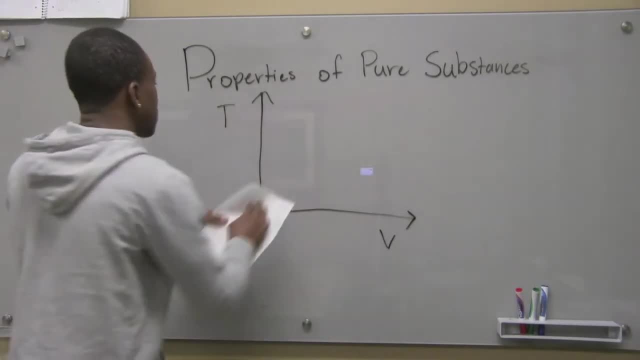 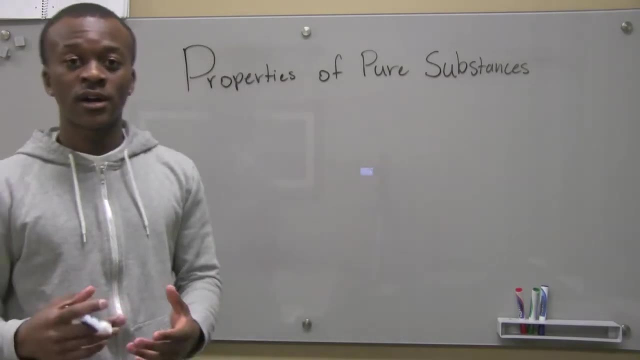 right. Actually, you know what? First, I'm going to talk about this To give us more of an idea of compressed liquids, saturated liquid gas mixtures, things like that, and superheated vapors. I'm going to take the. 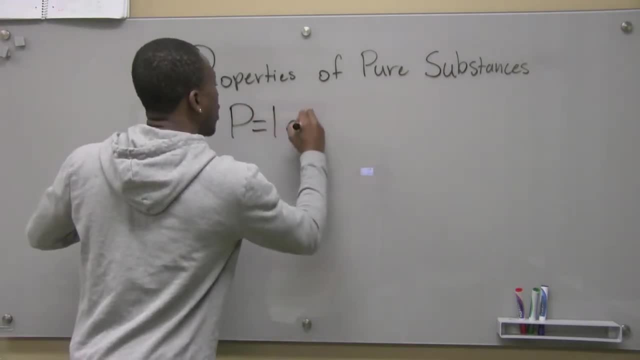 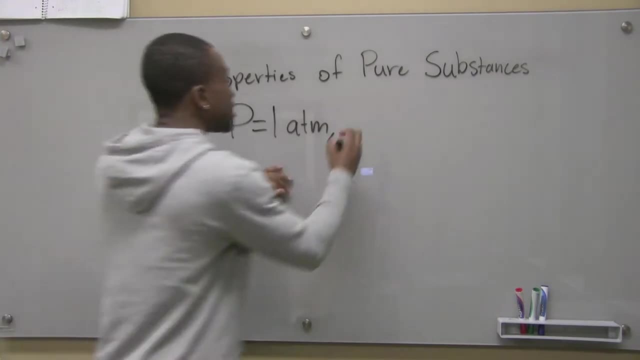 example of water. right, Let's say water at one atmosphere. I'm going to keep the pressure constant, but I'm going to vary with the temperature. So let's say my T for temperature. by the way, this is a unit of pressure atmospheres. So if I say my temperature is: 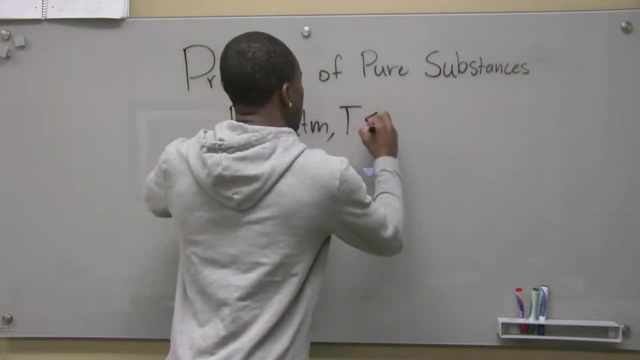 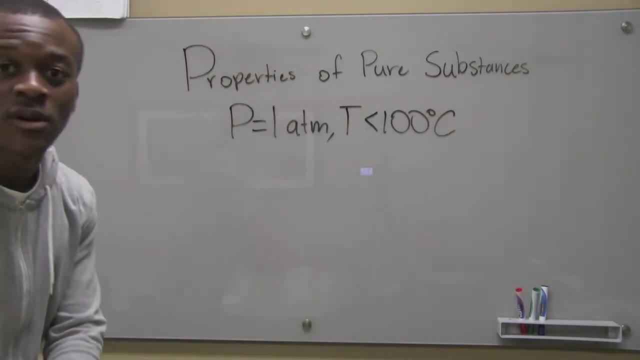 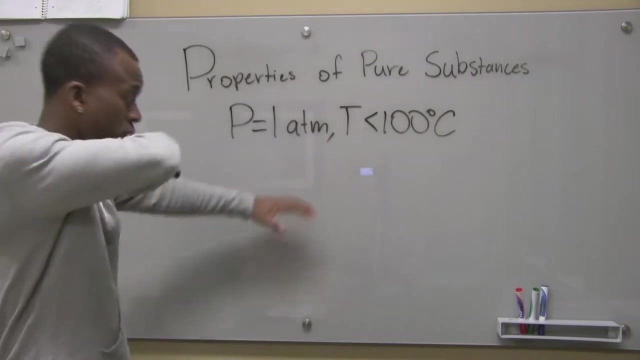 let me start off by saying my temperature is less than 100 degrees Celsius at one ATM. right, I'm going to have a compressed liquid, And this is because at one ATM, water's boiling point, or the saturation temperature for water, is 100 degrees Celsius. 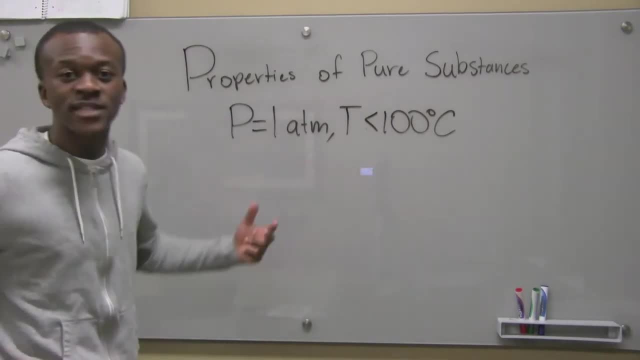 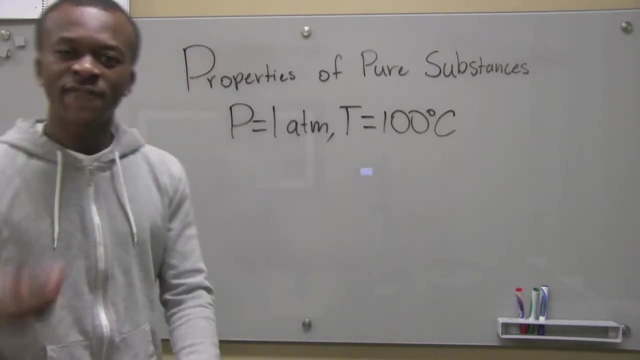 So if it's below that- 100 degrees Celsius at one ATM, it's not going to boil. If I now move on to say that my temperature is equal to 100 degrees Celsius, I'm going to have a compressed liquid. A few things can be going on here. I can either have a saturated liquid, which is like the water. 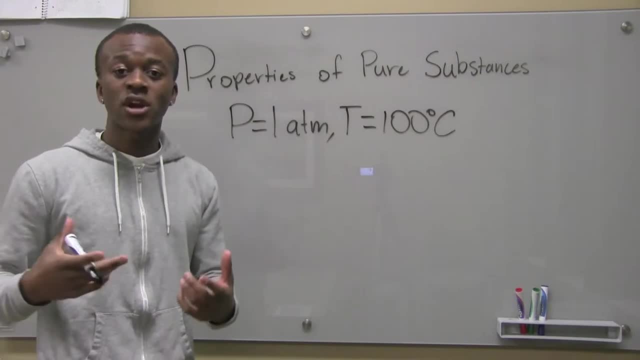 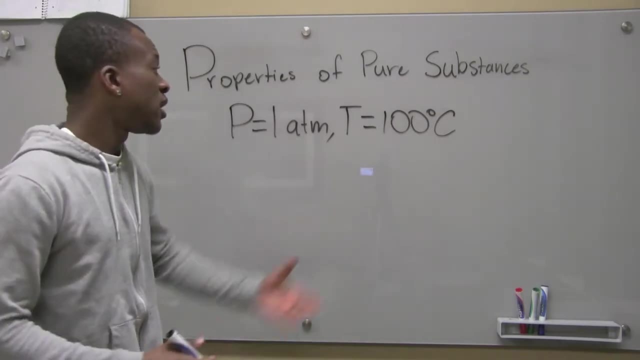 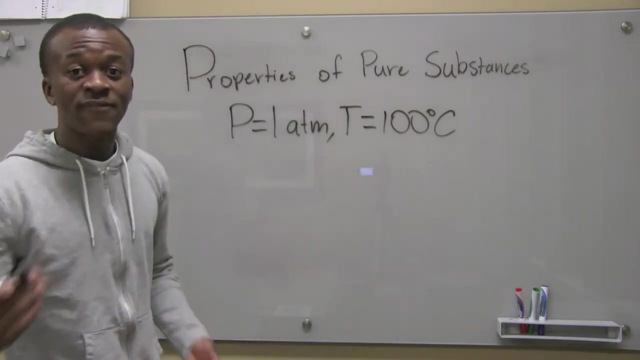 has just began boiling right And the first drop of liquid has just started boiling right Into a gas. I can have a saturated liquid gas mixture, or a saturated mixture, as I might call it, And that's where you have some liquid and some gas inside. or I could have a saturated vapor, And that's where 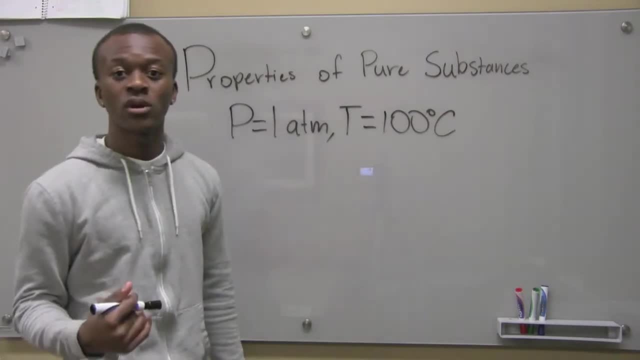 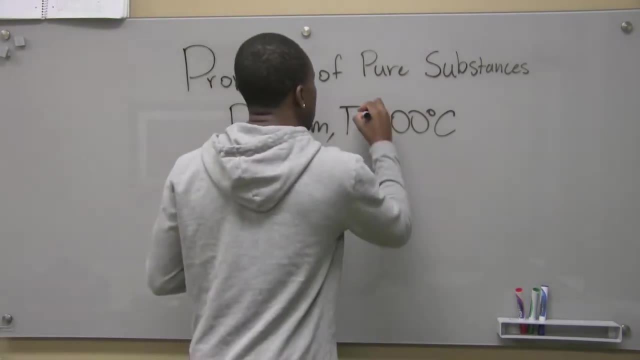 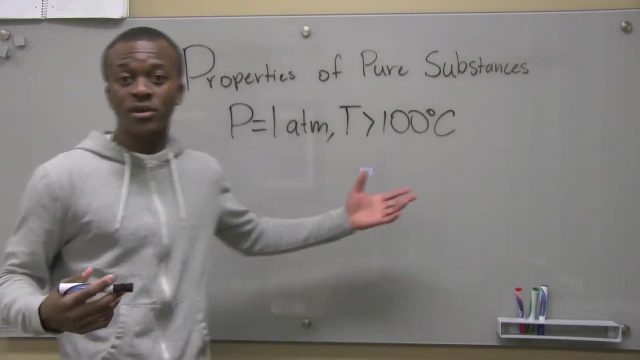 the last drop of water is just about to evaporate. I mean, it's just about to boil into a gas. right Now, if I'm at one atmosphere and I say that my temperature is greater than 100 degrees Celsius, I have a superheated vapor. This means that the substance, the water in this 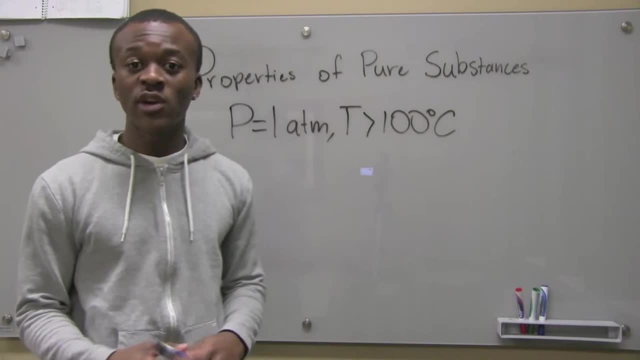 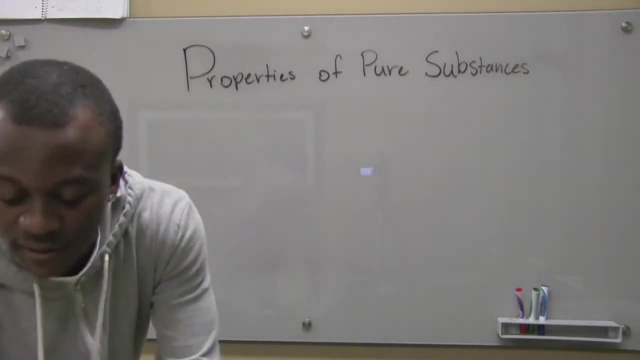 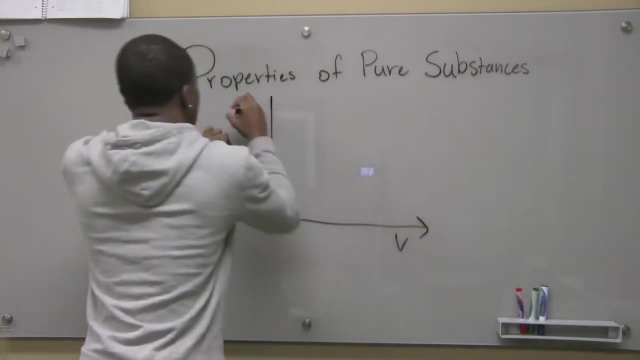 situation is totally gas. There's no liquid left. So I just wanted us to know that. Now I'm going to draw that TV graph I was talking about. Now I'm plotting temperature against volume or specific volume. right, Take your pick Now, based on what I just described. right, Let's? 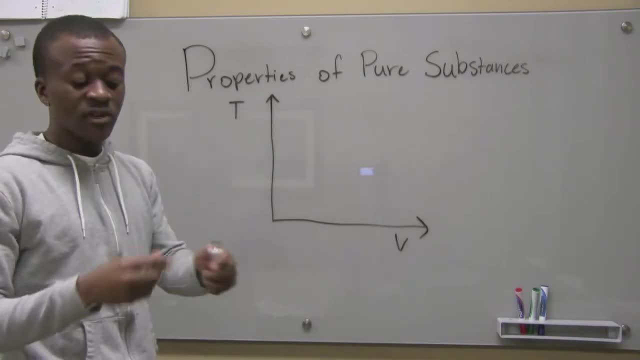 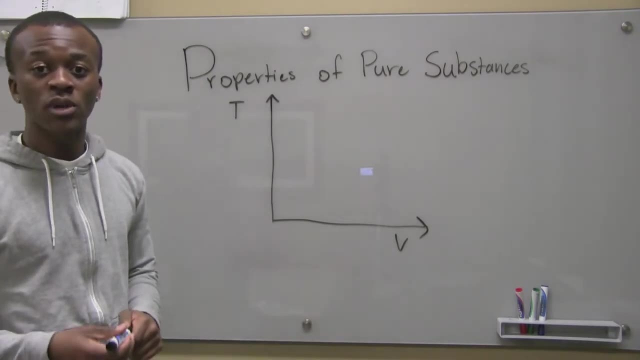 describe any phase changing substance. Water isn't the only phase changing substance I can give you. there's something called refrigerant 134A. I might substitute this by saying R134A, but that's just as valid of a phase changing substance as water is, So you're going to get something like this. 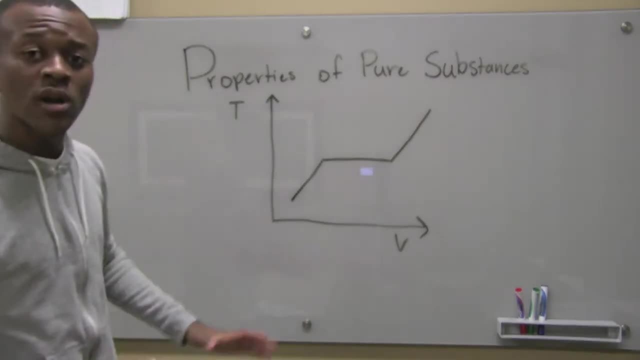 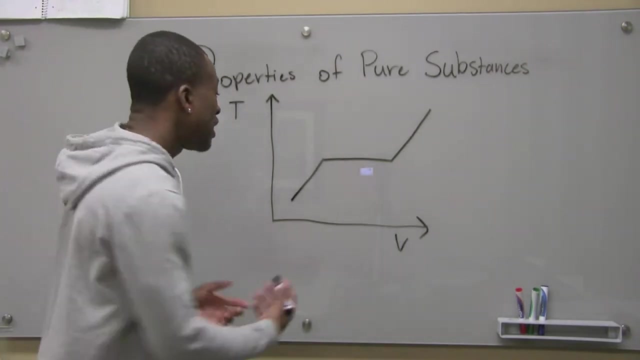 Now, what's going on here? Now the water. I'm heating it up right As I first start. let's say, I start with a liquid, a compressed liquid. right, I'm heating that water up. right, As I'm heating it up. 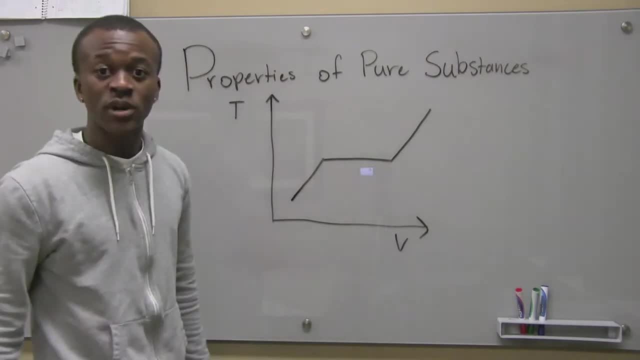 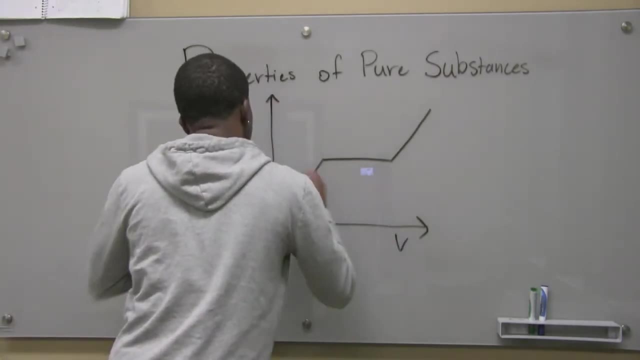 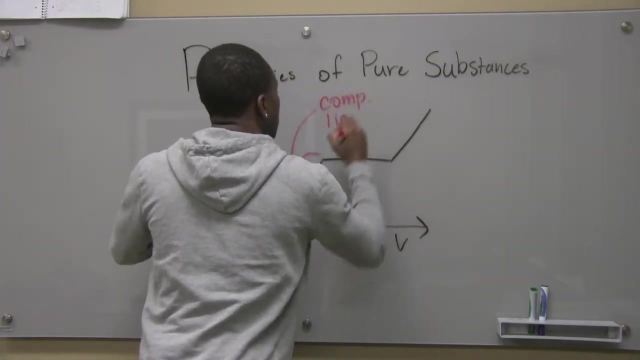 what is increasing. Both the temperature and the volume are increasing at this point in time. What is a compressed liquid right? So this is the compressed liquid state. I'm just going to write, Just to abbreviate. That's the compressed liquid right there. Now, when it gets to this point, right. 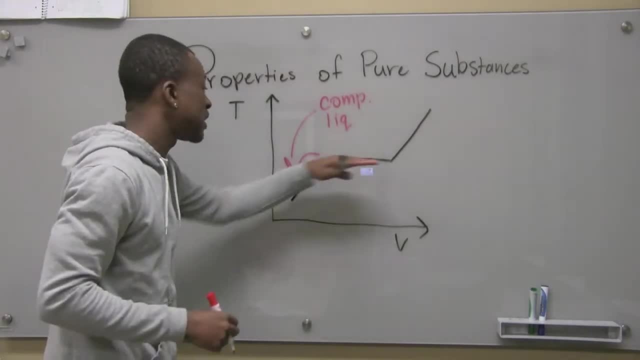 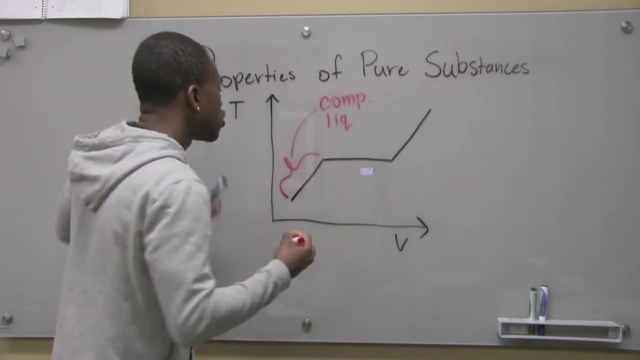 here, right, Where it just starts boiling, right. First of all, let's look at this line. What's a constant here? Temperature is a constant right, While volume is still increasing- right, A specific volume. So what's going to end up happening is this is going to be our saturated liquid point. 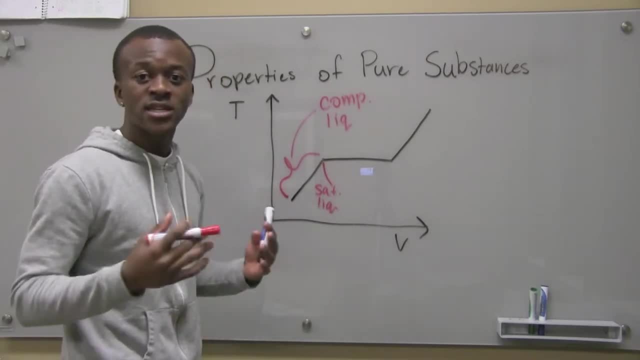 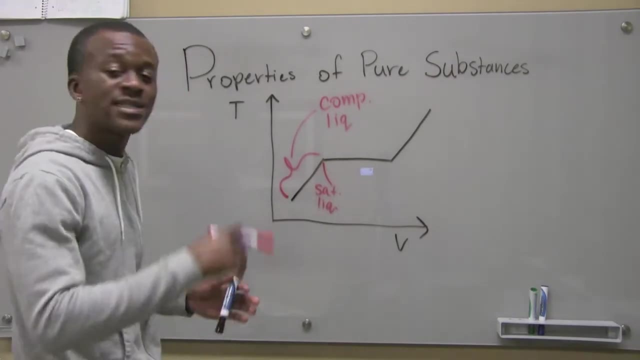 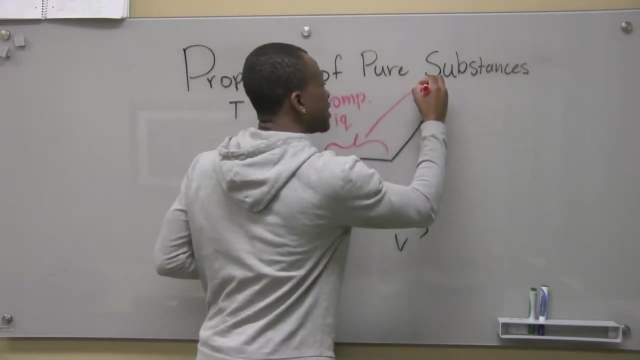 Now, after this thing reaches saturation, it doesn't just stop, It doesn't just keep increasing in temperature, It stays constant at temperature until it reaches. Now, here, we're going to have boiling, right, Boiling is going to take place and we're going to have a. 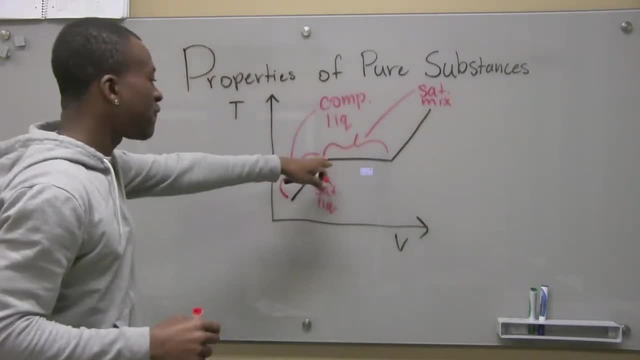 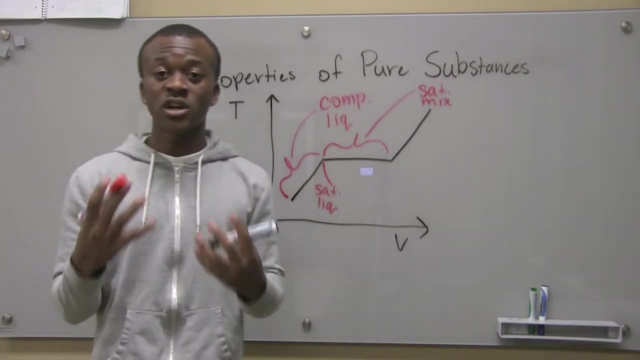 saturated mixture. From here, on this straight line, we have a saturated mixture And this is just where the liquid- compressed liquid water- has become a superheated vapor. So you're going to have part of it is going to be a superheated vapor, Part of it is going to be. 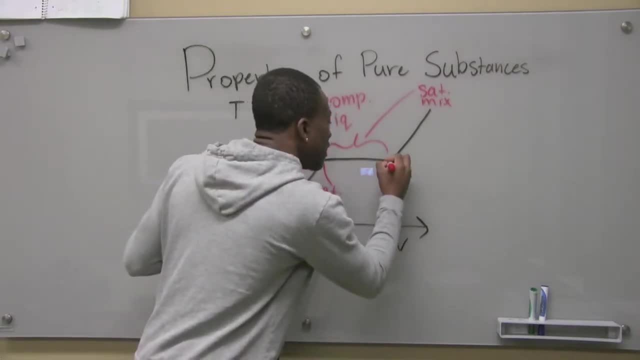 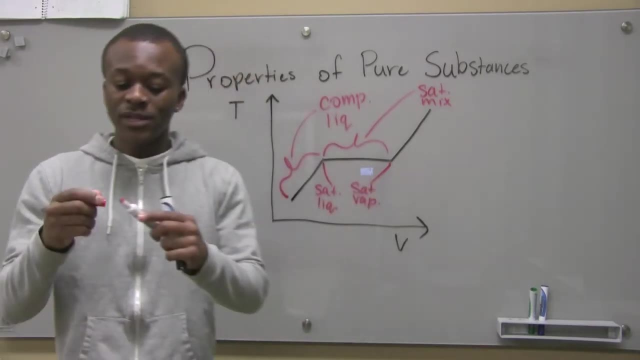 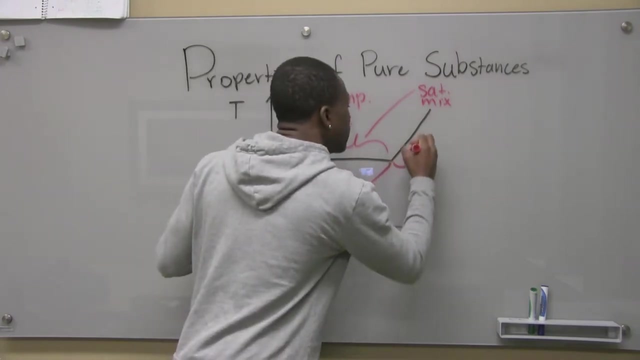 compressed liquid. Now, once we reach this point right here, this is going to be our saturated vapor. This is the point where, as I said, the last drop of water is just about to boil. So that's what we know is going on here. Now, this part, intuitively we can say, is a superheated vapor. 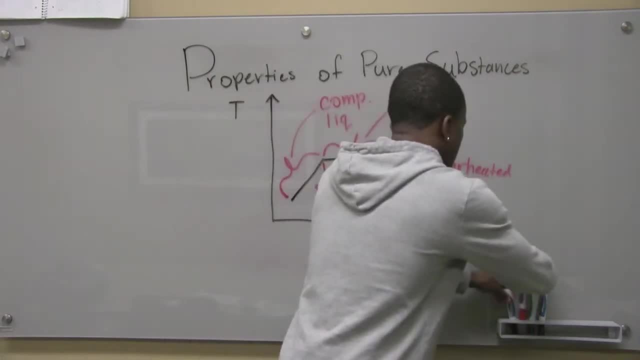 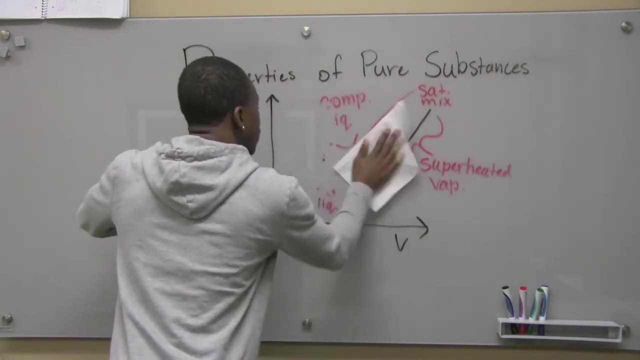 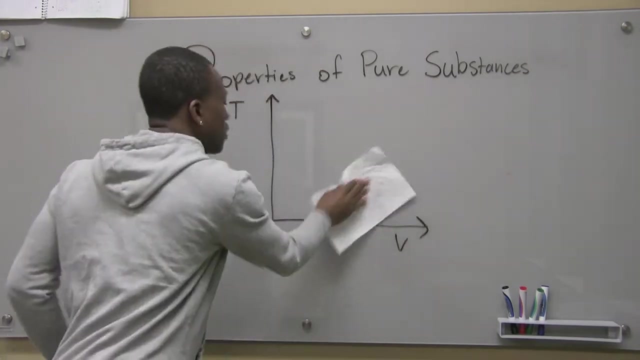 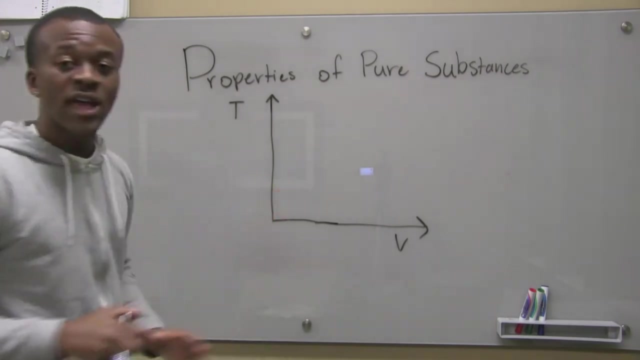 Now keep this graph in mind. We can do this to remember that this is a constant pressure line. right Now, let's say I were to choose a pressure that I'm going to analyze water at Now, drawing that same constant pressure line. I'm not going to specify at every single point. 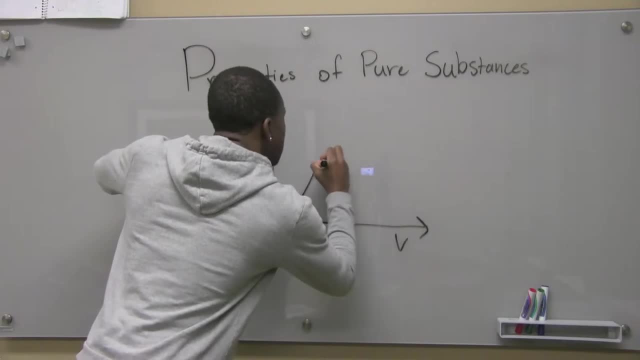 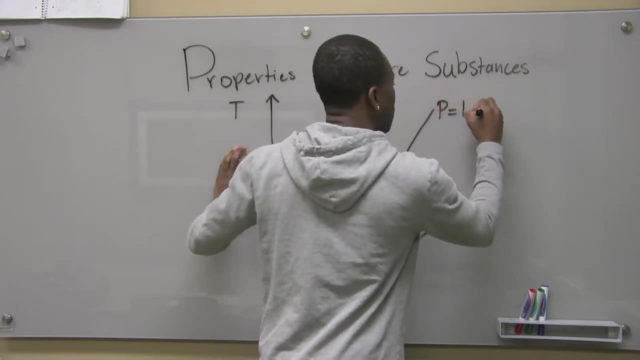 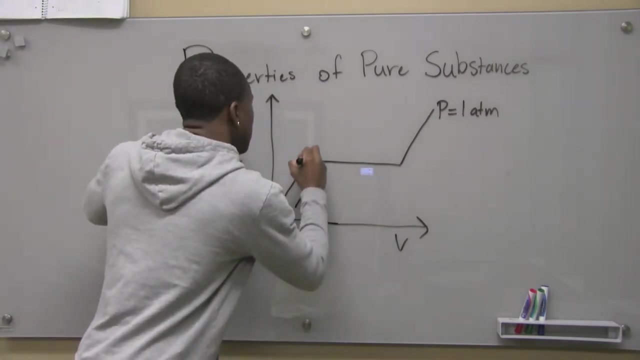 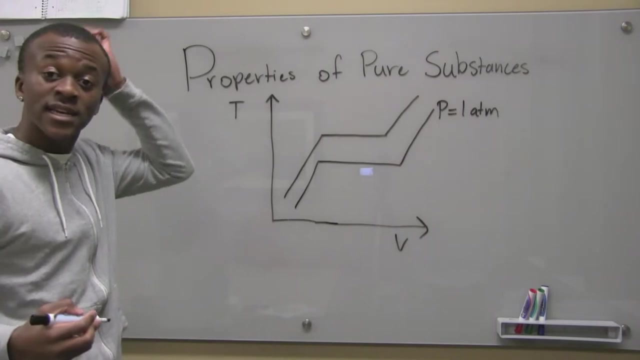 what's going on here, because you guys already know. So let's say: I chose to do this. All right, let's say I choose that P to be one atmosphere. Now let's say I choose a slightly higher P. right, I'm going to get a graph that looks something like this. right, Let's say that's. 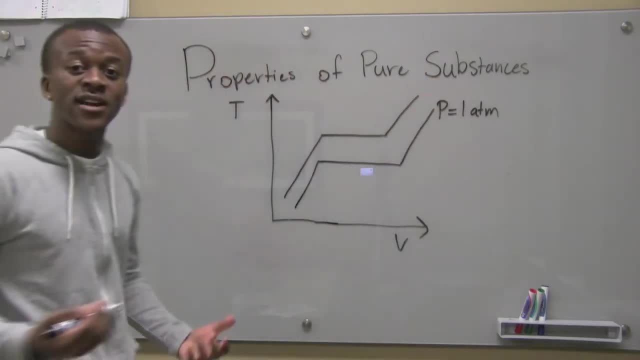 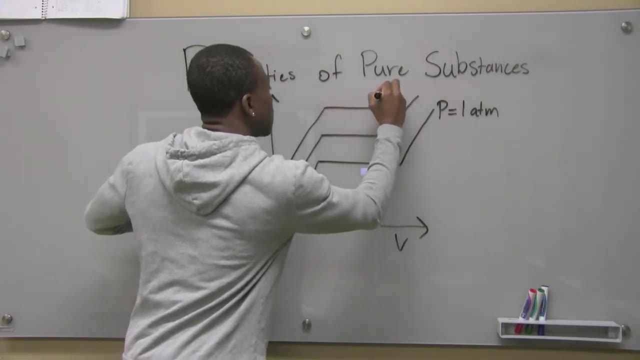 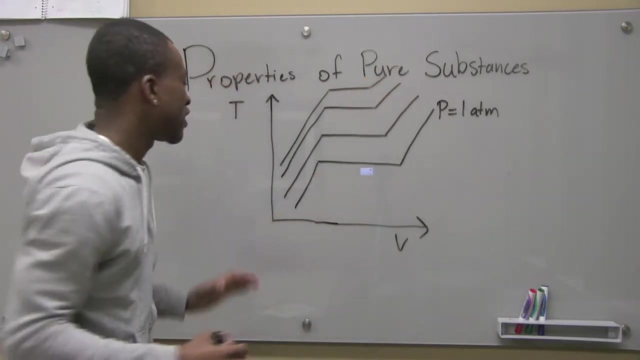 two atmosphere. All right, to be honest, just keep in mind that it's higher than one. Now, let's say, I keep doing that, I'm going to get something that looks like this, something that looks like this, And you guys can sort of get the point right. If I fill these in right, I'll get something that. 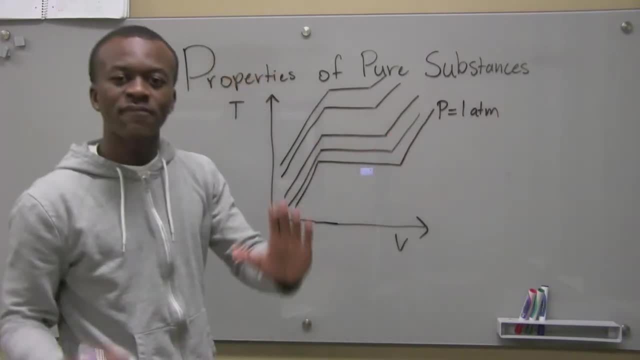 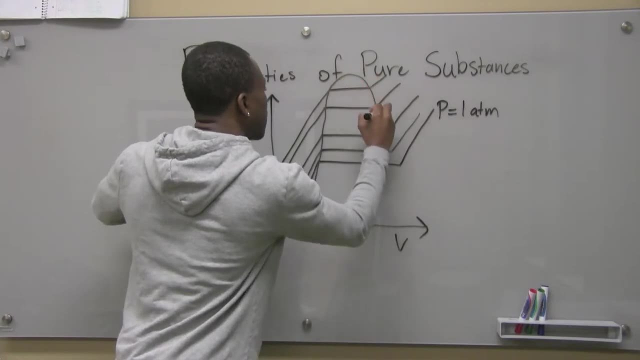 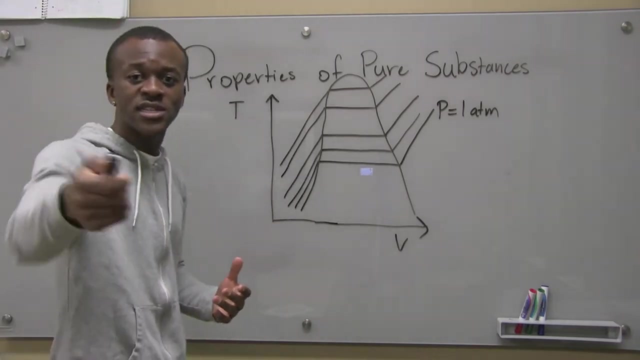 looks like this And it sort of makes like a dome. once we can connect these points- And excuse my drawing because it's not to scale, but we can sort of get a type of dome And we get something that like this: Now, intuitively, based on what I have just said, we can see that this line is the 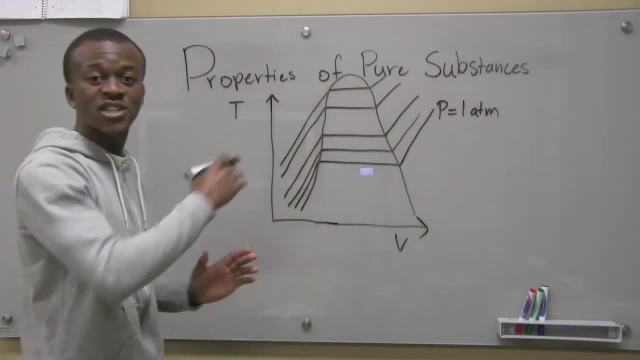 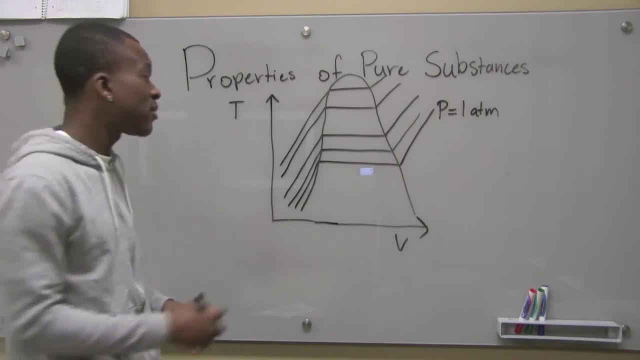 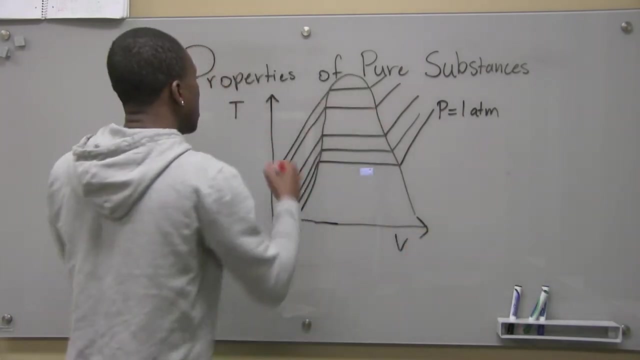 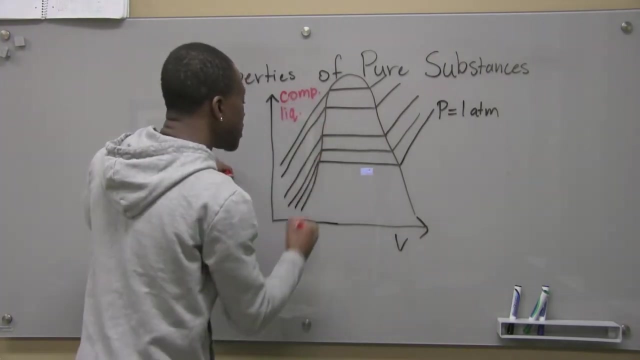 compressed liquid line. right, This point is our saturated liquid point. This is the area of a saturated mixture. This point is a saturated vapor and this is a superheated vapor. Now what's going on here? On this side of the dome, we have a compressed liquid. This line denotes a saturated. 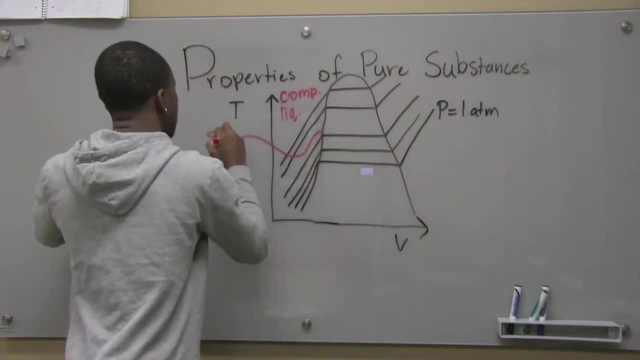 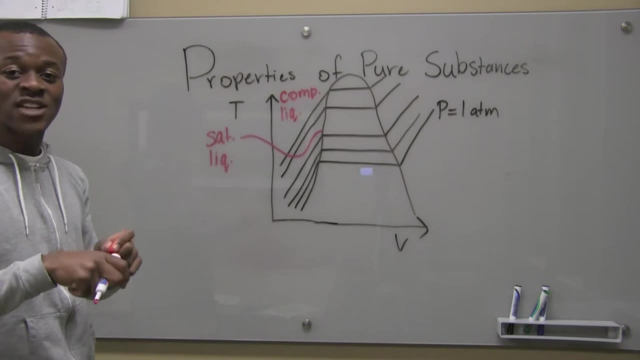 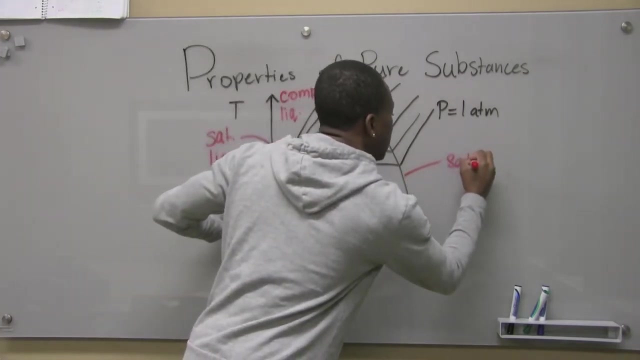 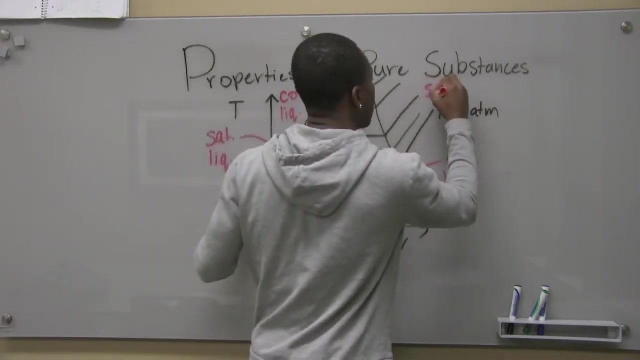 liquid. Now, any time we're inside of the dome we're going to have a saturated mixture. So this has Saturated mixture. just means that we have liquid and vapor inside. This is the saturated vapor line And then we have the superheated vapor area- everything on the right side of the dome. 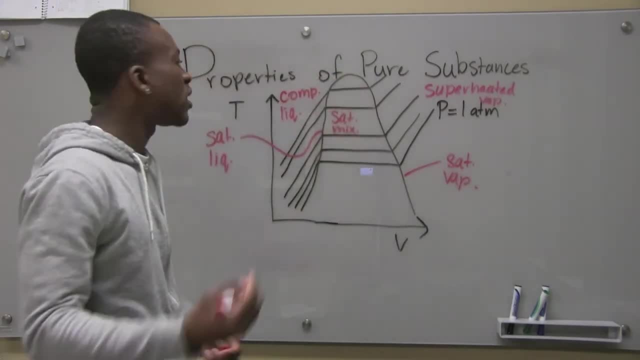 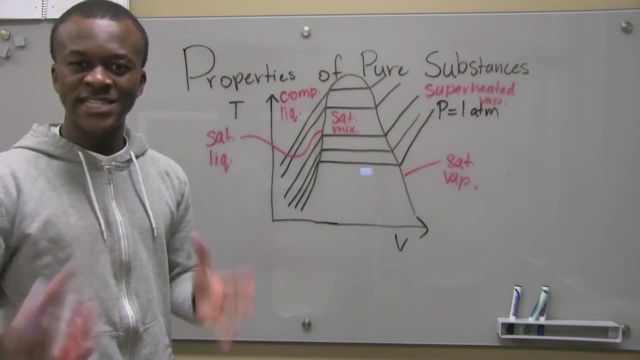 Now you might be asking: what happens at this point right here? What's going on? This is something called the critical point. That's just where the phases are sort of indistinguishable. So I mean, just keep that in mind, It doesn't come into play too much. 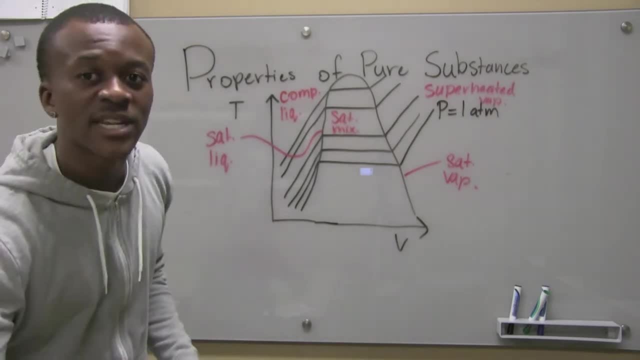 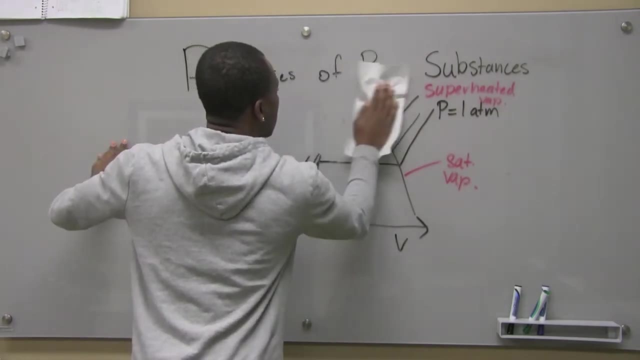 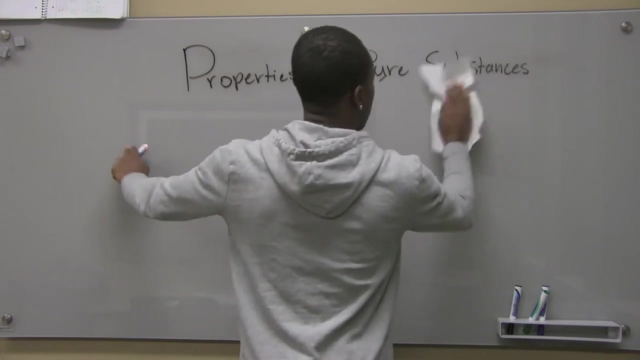 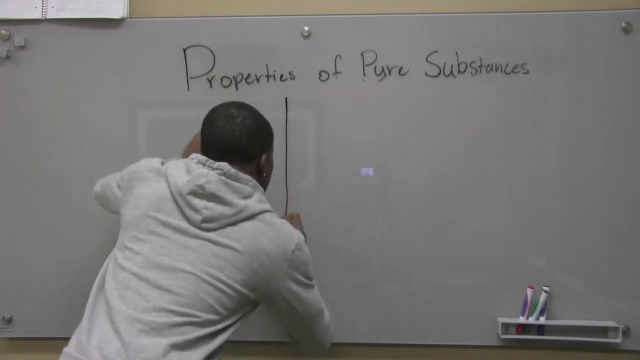 Well, at least I don't think it's going to come into play too much, but just keep that in mind. It's something called the critical point. Now I want to show you guys something else. If I'm to draw something called a PV diagram, right? 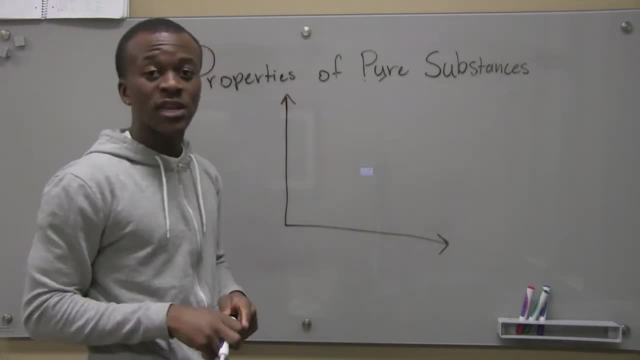 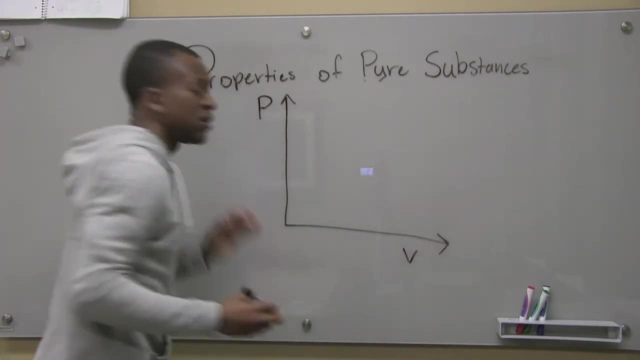 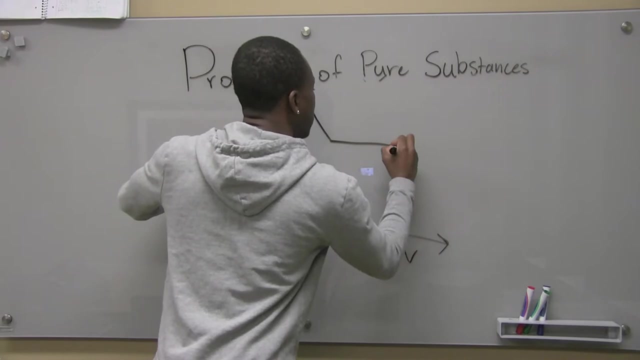 I just drew you guys a TV diagram where I was plotting temperature against volume or specific volume. Now I'm plotting pressure against specific volume. Now what we're going to get here is something that looks sort of like this: Now what's going on here? 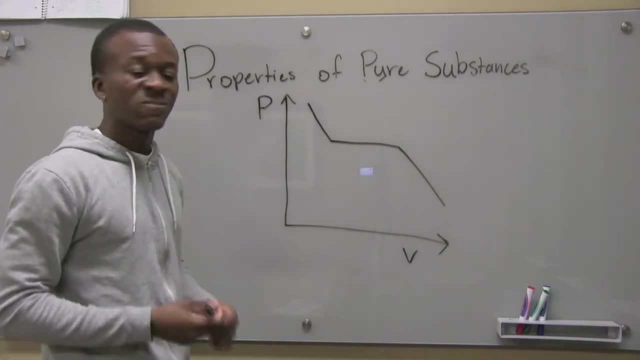 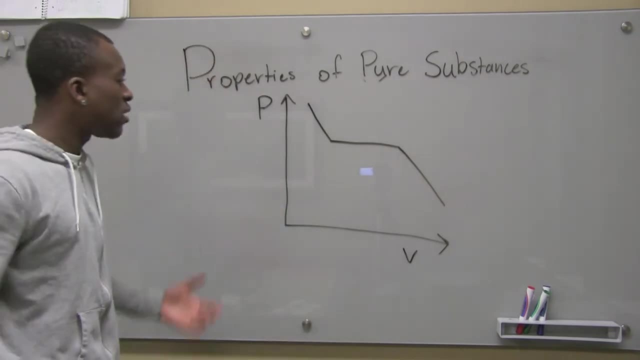 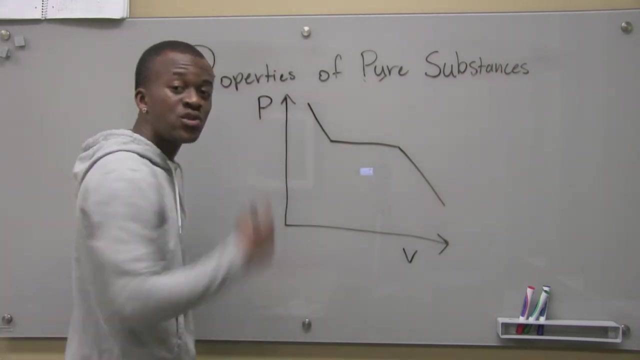 Remember, I have a constant temperature line right, Just as I had my constant pressure line before. Now this becomes a constant temperature line because I'm plotting pressure against volume. Now what's going on? This shows you that, as you're at a constant temperature, as you decrease the pressure. 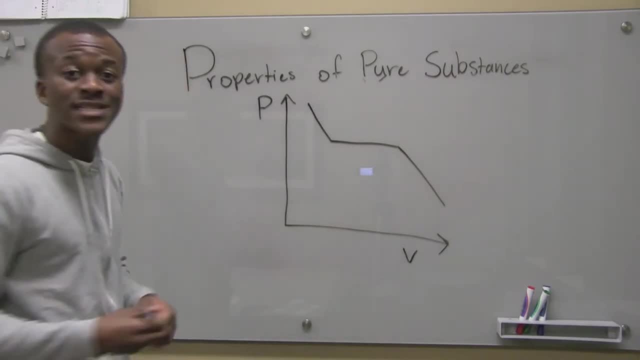 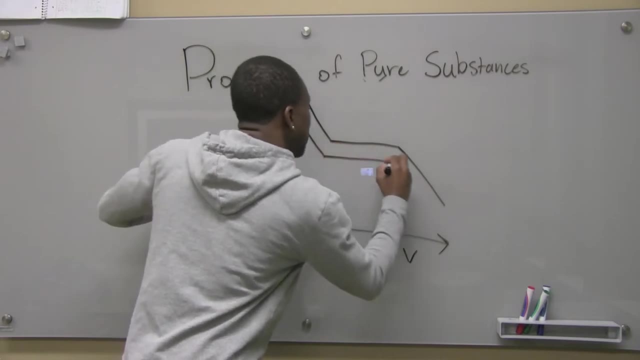 your substance wants to start boiling. So now, if I'm to do that same sort of arrangement that I did before, right, I'm going to end up getting something like this: Let's say, I took at a lower temperature, right, That should actually come like this. 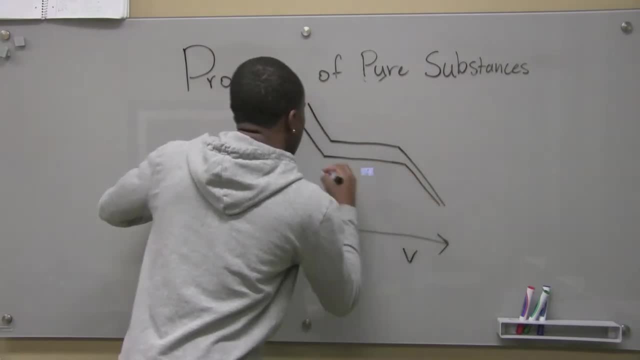 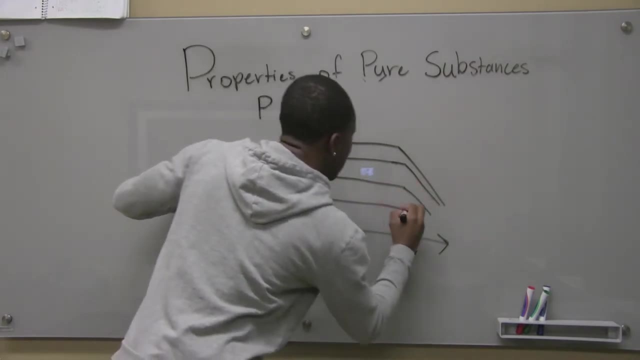 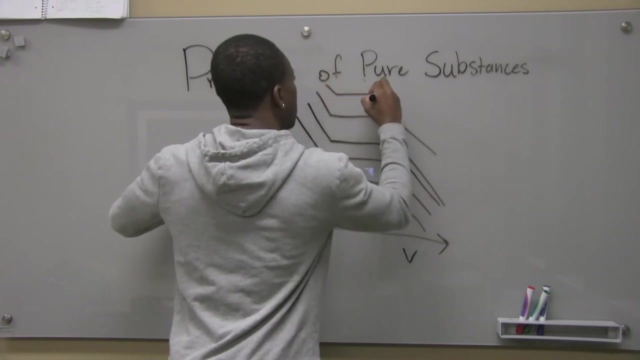 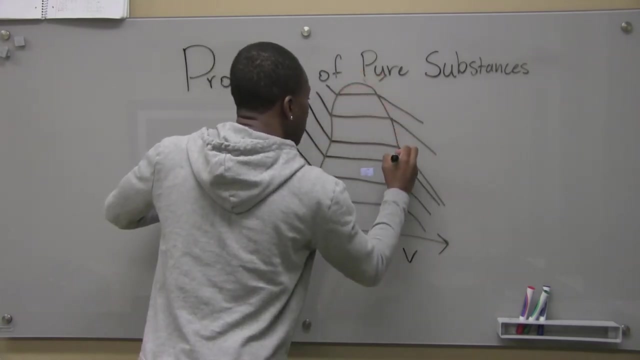 Okay, And at an even lower temperature. an even lower temperature, and you guys get the point. So we're going to end up having something like this, and then we can connect the dome. Excuse, again, my drawing is not to scale, but it looks something like this, right? 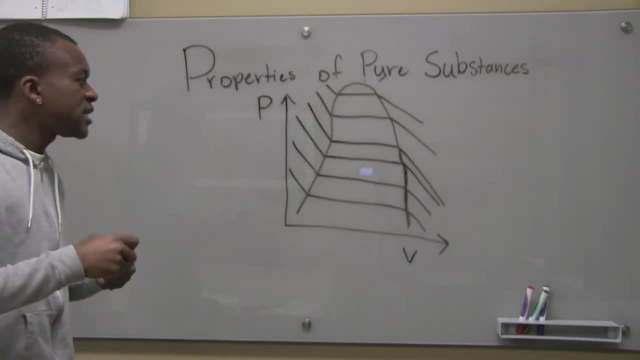 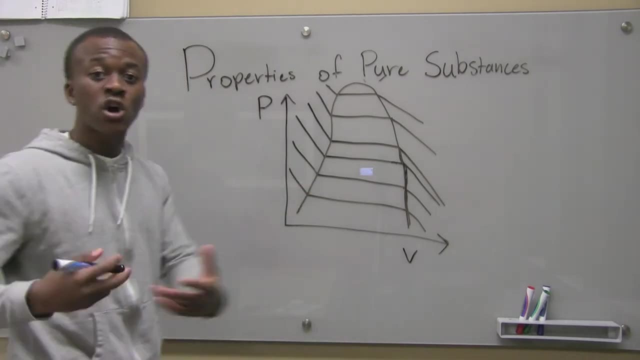 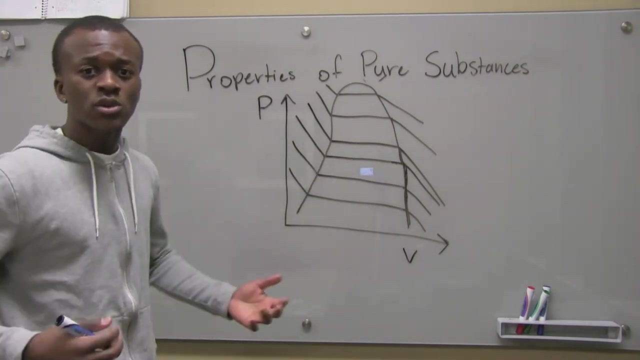 It's just a dome basically. Just keep that in mind. So we can see that temperature and pressure are sort of opposites. Keeping the temperature the same and decreasing my pressure causes my liquid to boil. Keeping my pressure the same and increasing the temperature causes my liquid to boil. 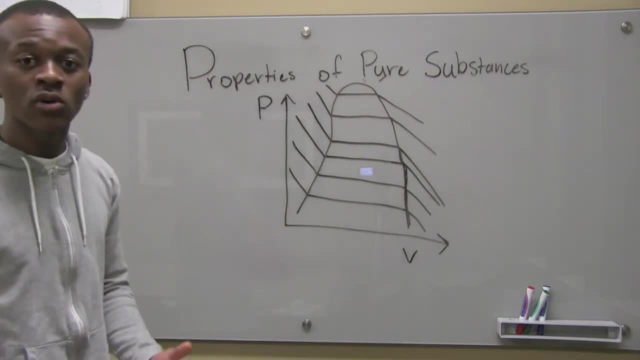 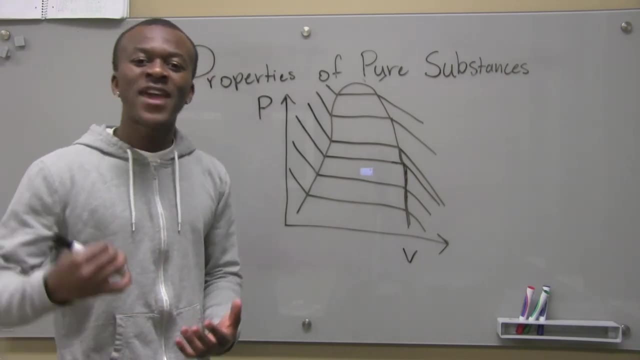 So it's sort of the same thing. Now we're going to sort of get into something called quality. right, Just to give you a sort of brief summary, quality is just sort of it favors your vapor over your liquid, Your compressed liquid. 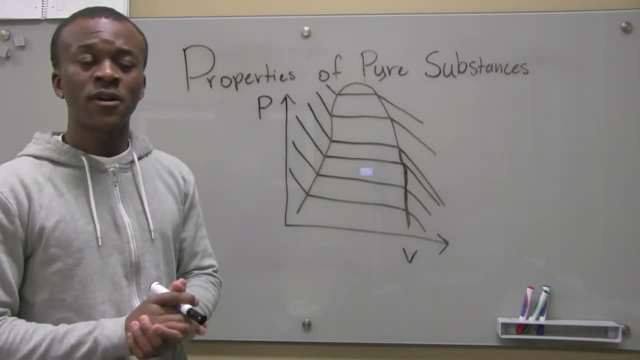 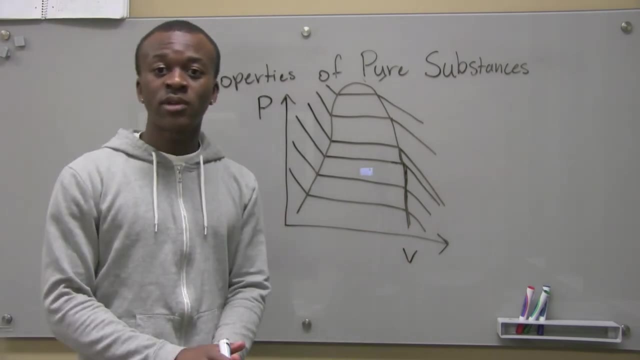 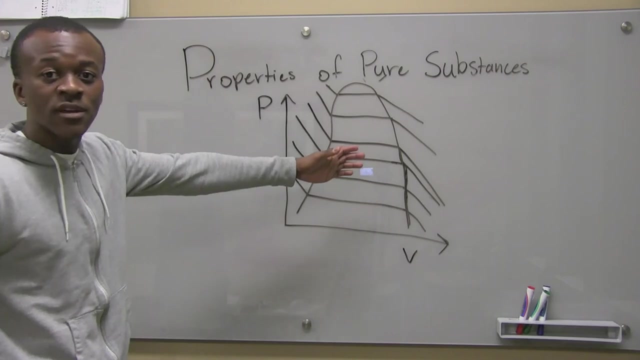 And by that I mean quality, is basically the percentage of superheated vapor that you have in a mixture. Generally, quality only comes into play in a saturated liquid vapor mixture. I don't know, I can't talk, But it only comes into play there really, because what do you think your quality is going to? 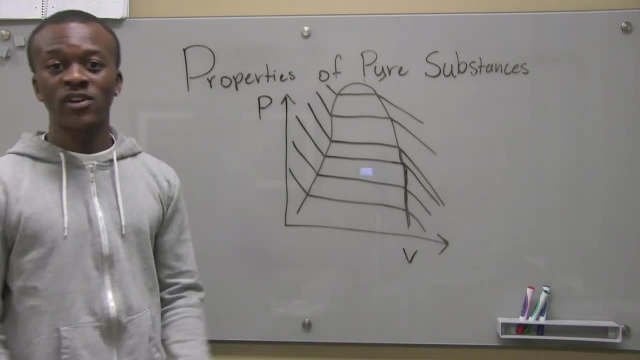 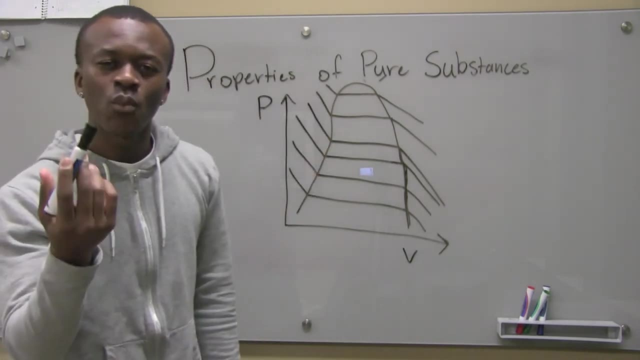 be for a compressed liquid. What percentage of superheated vapor do we have in a compressed liquid? Zero, right. What about at our point of where it's like a saturated liquid? What do you think the quality is going to be? It's going to be zero, right. 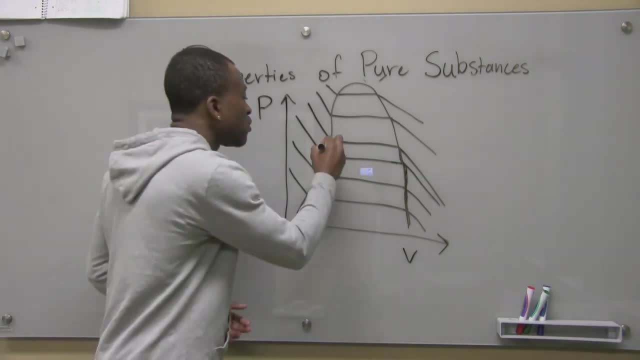 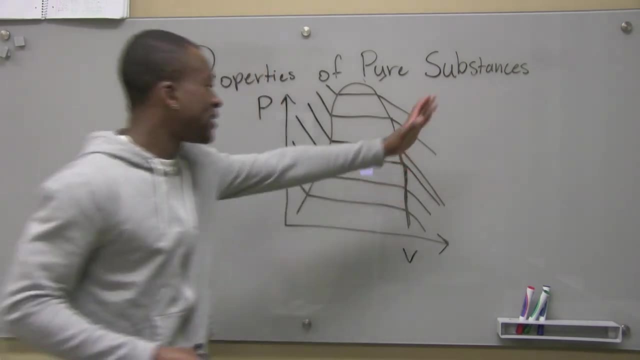 And quality. you can say like zero percent, right, As we move here, it's going to increase from zero to a hundred percent when it reaches the saturated vapor state, and we're going to then have a superheated vapor where the quality is always going to be. 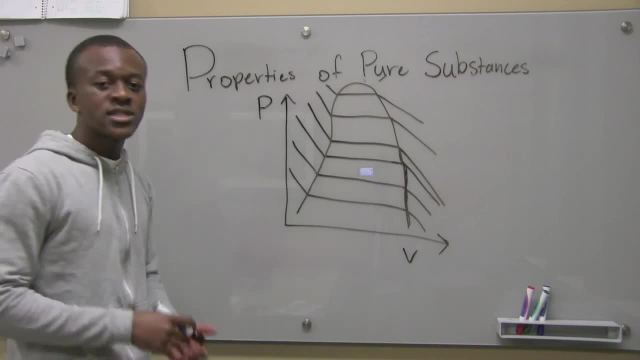 Like quality doesn't really come into play there. So stay tuned And we'll learn a little bit more about this. I hope you guys enjoyed this video. Thank you.